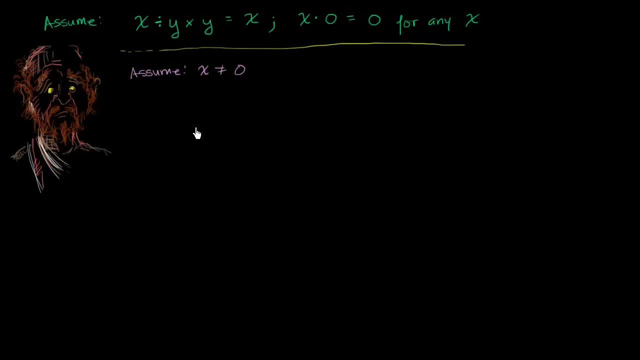 what x divided by 0 should be. how I should define it is just assume that it's defined and then come up with any results that I might, or maybe I'll even be able to solve for it. So let's say that x divided by 0. 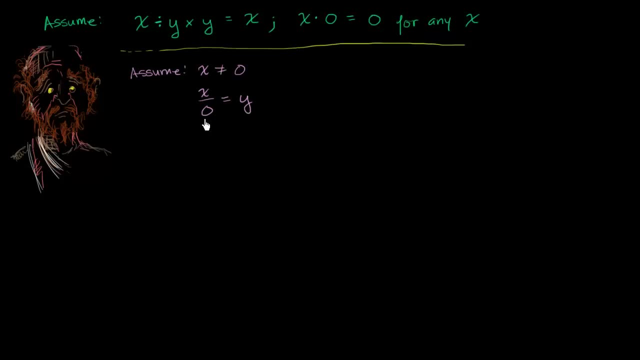 is equal to. let's say that it is equal to y. Well, I'll use a different number just to not get you confused with this up here. Let's say it's equal to. let's say that it is equal to k. 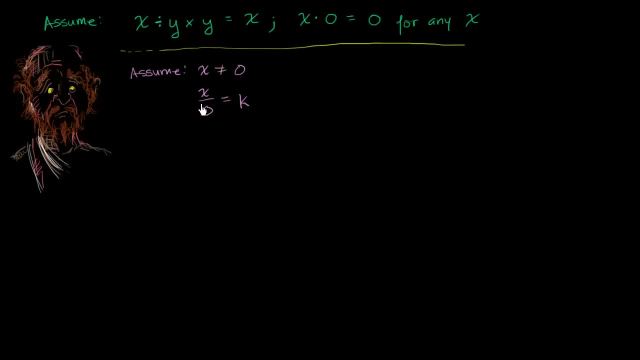 Well, if this is true and if we're dividing, if we're defining what it means to divide by 0, then we're assuming that if we multiply by 0, we need to get our original number right over here. This is something that we are not willing to contradict. 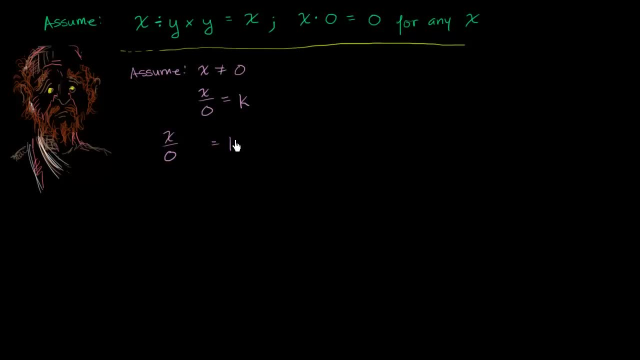 So let's see what happens: x divided by 0 is equal to k On the left-hand side. I'm going to divide by 0, and then multiply by 0. Well, if I do, if two things are equal. 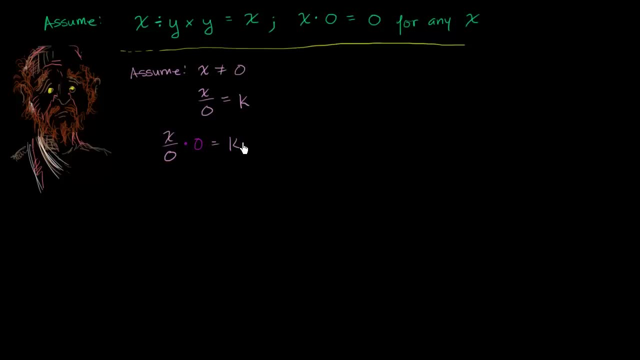 and I do it on. if I do something to one thing in order for them to stay equal, I have to do it to the other thing. This has to be equal to that. I have to multiply both the left and the right-hand sides by 0.. 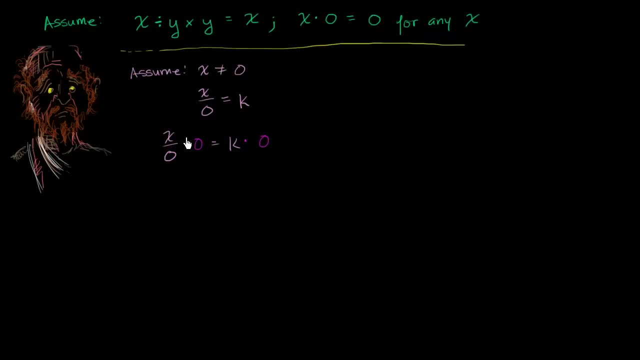 Well, by this assumption that I'm never willing to give up, this left-hand side right over here must be equal to x, This must be equal to x. And by this assumption right over here that I'm not willing to give up this right-hand side right over here, 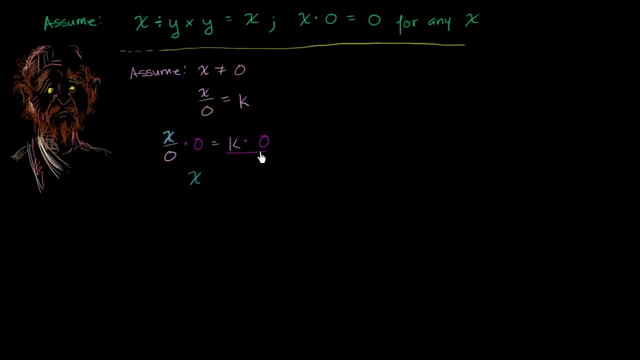 must be equal to this right-hand side must be equal to 0. But I just hit a contradiction. I assume that x does not equal to 0, and now I'm being forced to say that x equals 0. And I'm not willing to give up the idea. 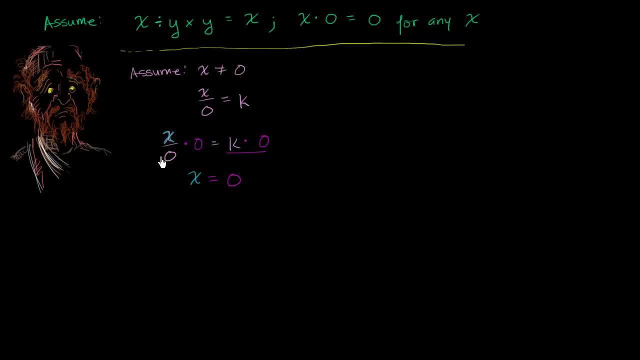 either of these ideas. I'm not willing to give up the idea that if I'm defining what it means to divide by 0, or if I'm defining what it means to divide by anything, that if I then multiply by that something, that I should get my original number. 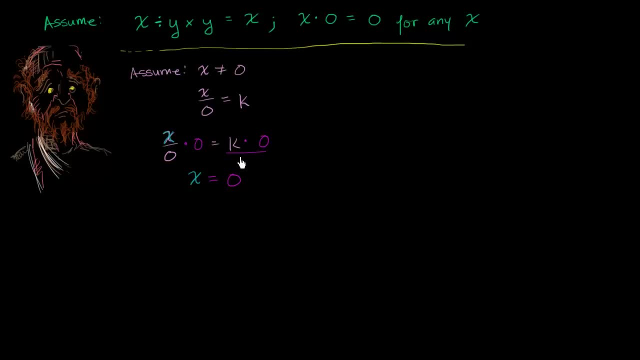 And I'm not willing to give up the idea that anything times 0 is 0.. So, out of all of these things, the only thing that I can give up, the only thing that I can give up is this, right over here, And I'll say: well, 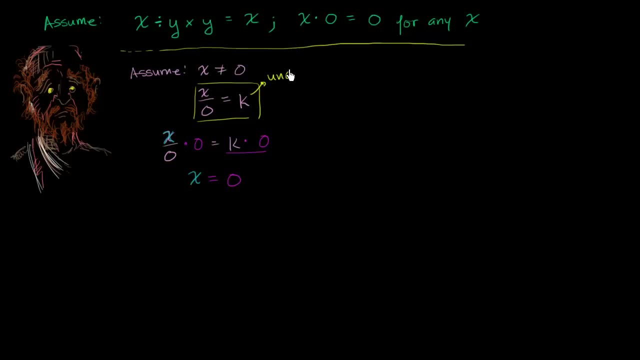 I guess k will have to stay. k will have to stay undefined. This whole contradiction happened because I attempted to define what x divided by 0 is. Now, with that out of the way, you're like? well, okay, this was the situation when x does not equal 0. 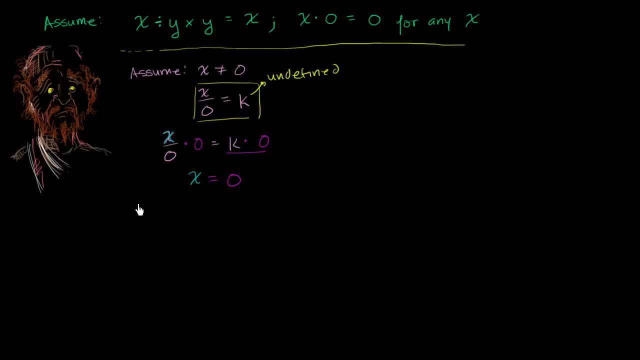 But what about when x does equal 0?? So let's think about that for a little bit. Let's think about that a little bit And once again I will try to define it. So I will assume, I will assume that 0 divided by 0,. 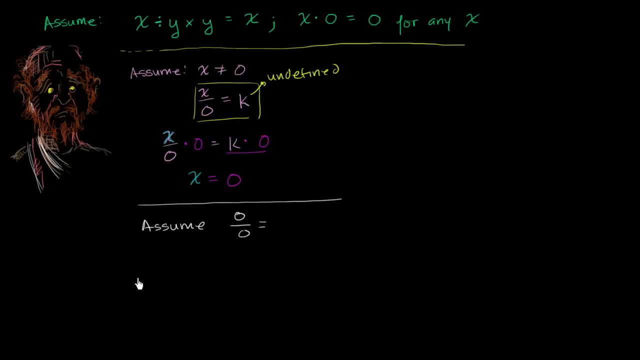 is equal to some number. Well, once again, let's just say it's equal to. let's say it's equal to k again. And so, once again, we're going to try to do the same logic, So I'm going to rewrite it again. 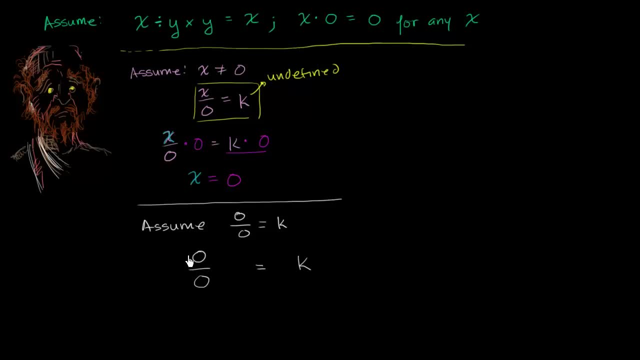 0 divided by 0 is equal to k, And actually let me color code the 0s. So that's a magenta 0.. This is a blue 0 right over here, And once again I'm not willing to give up the idea. 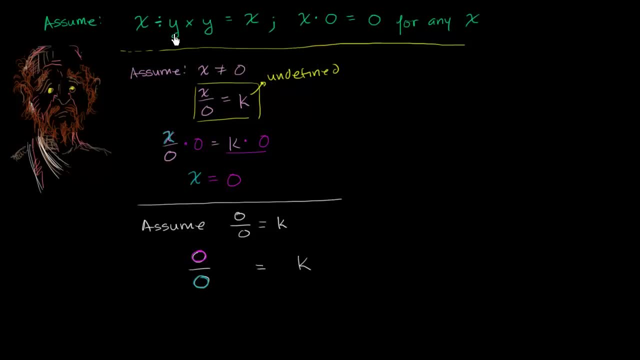 that if I start with a number x, I divide it by something over which division is defined and then I multiply. I multiply by that something that I should get my original x again. Can't give this up. Otherwise it doesn't seem like a good definition for division. 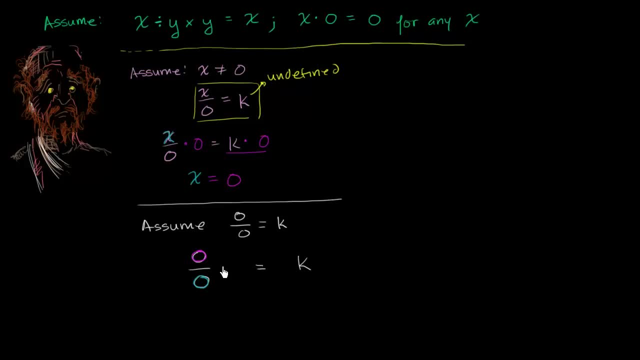 So what I'm going to do is I'm going to multiply the left-hand side times 0.. And by this property that I'm not willing to give up, the left-hand side should simplify to this magenta: 0.. This should simplify to this right over here. 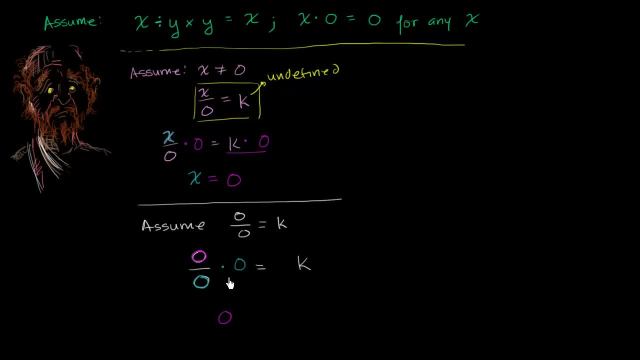 But once again, anything I do to one side of an equation, in order for the equation to hold true, I need to do the other side of the equation. If these two are equal beforehand, any operation I do to this in order for it to still be equal. 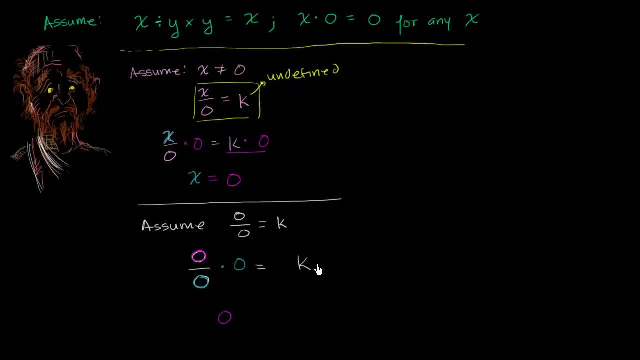 I need to do to that. So let me multiply the right-hand side. Let me multiply the right-hand side by 0. So on the left, I get 0.. I just get this magenta 0.. And on the right, I get. 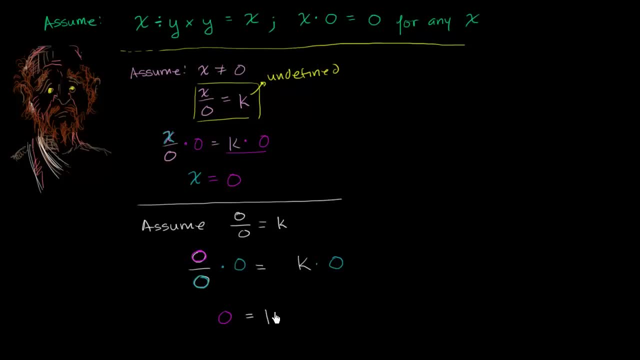 I could just write a 0 here, but I won't simplify it. I get k times 0.. k times 0.. Well, this I see right over here. this actually is not a contradiction. This is actually true. This is actually true for any k. 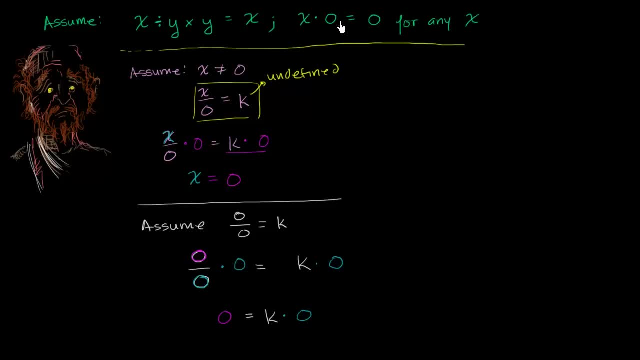 This is actually one of my core assumptions that I made in my mathematics, that I'm not willing to give up. So this is true and let me write it bold: This is true, true for any. This is true for any k. It's not a contradiction. 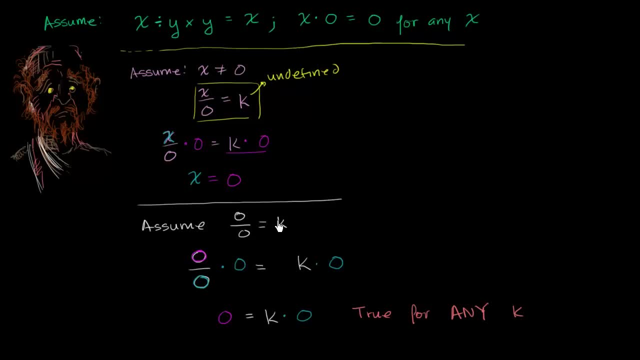 but the problem here is: I wanted to come up with a k. I wanted to almost solve for a k. It would have been nice if this turned out to be 0, or if this turned out to be 1, or if this turned out to be negative 1.. 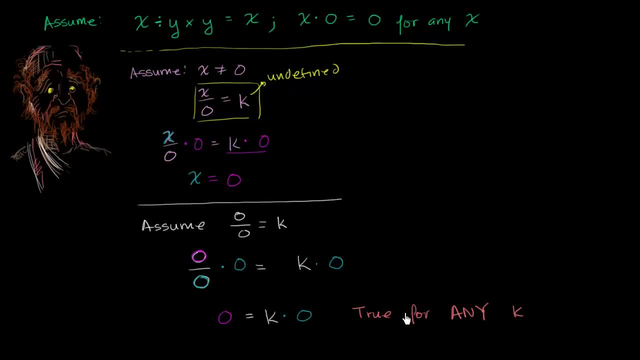 But now I'm seeing that, given the assumptions up here, this could be any. This could be absolutely any k. I cannot determine what k this should be. This could be 100,000.. This could be 75.. It could be anything. 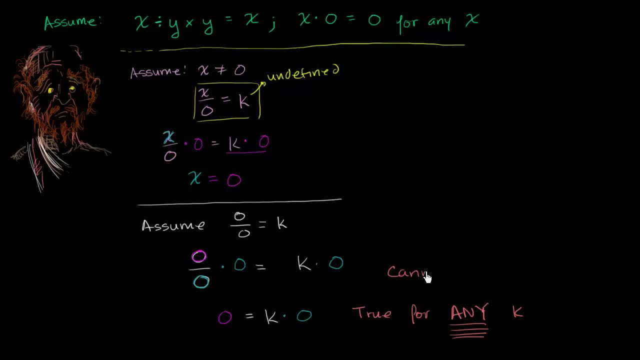 True for any k. I cannot determine what k this should be, And that's why, when you get a little bit more nuance in early math, people will say, well, 0 divided by 0, well, we don't know what that's going to be. 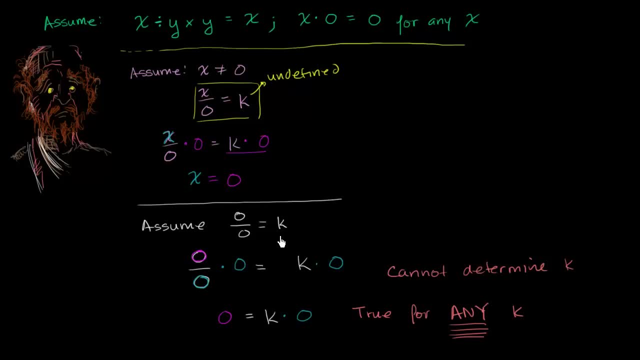 There's no consistent answer there, so we're just going to call it undefined. There's no good answer. that seems to be better than any other answer. But now we see a little bit of nuance here: 1 divided by 0, you just couldn't define it. 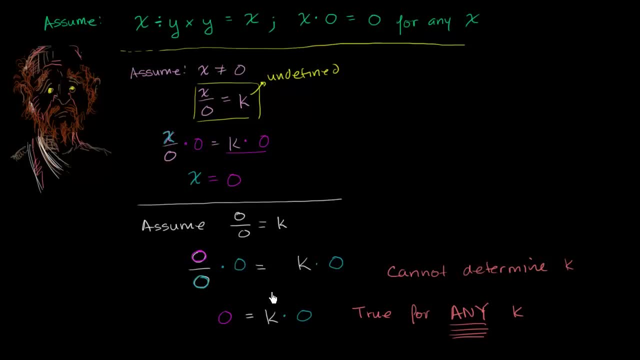 It led to direct contradictions: 0 divided by 0, it could be anything. You can't determine it, And so that's why, as you get to higher level of math- and you'll often hear this when you take a calculus course- 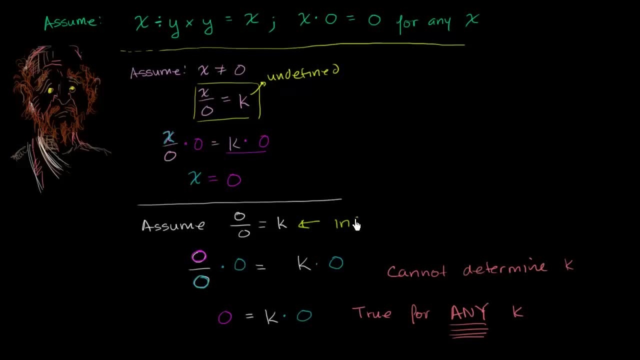 we say that 0 divided by 0 is indeterminate. Indeterminate. 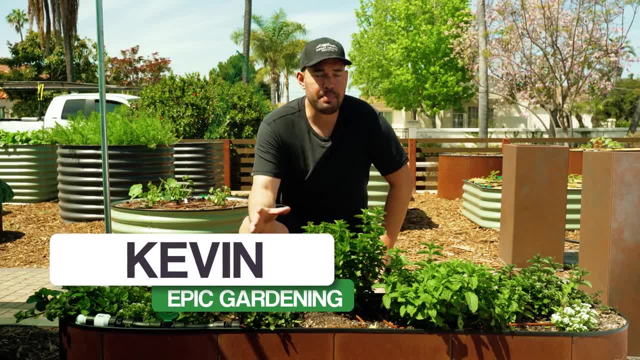 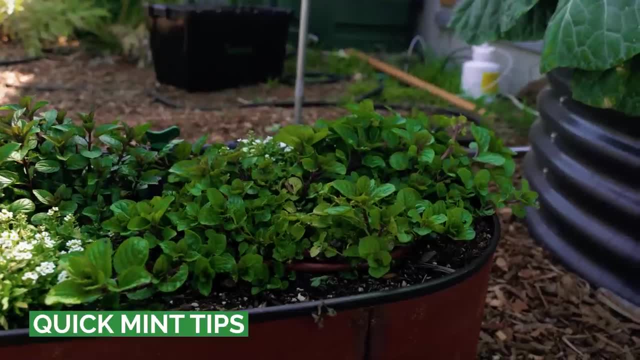 In today's video, I'm going to show you how to grow one of the most popular herbs of all time- mint- without letting it take over your garden. I have a ton of different varieties of mint in this raised bed which I'm excited to share with you. But first, 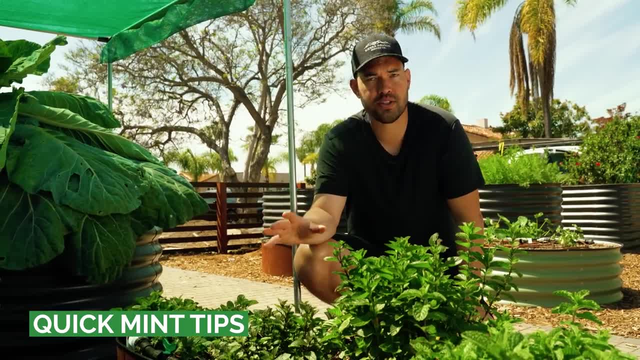 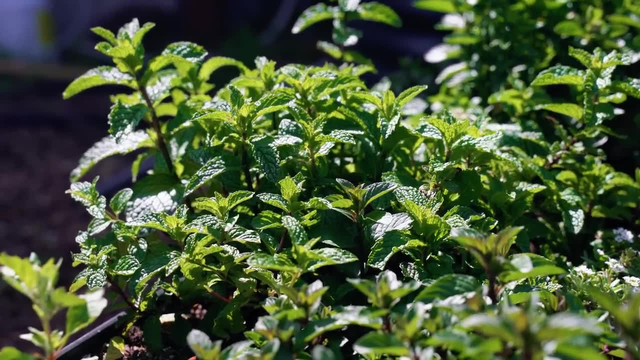 just a couple of quick tips on mint care. It's a simple plant to grow, guys, Very simple. You want ample light, not too much, though It can be in a little bit of shade. You want a moist soil that is rich in organic matter. 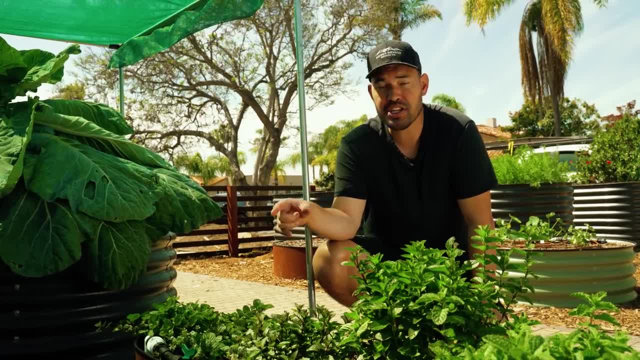 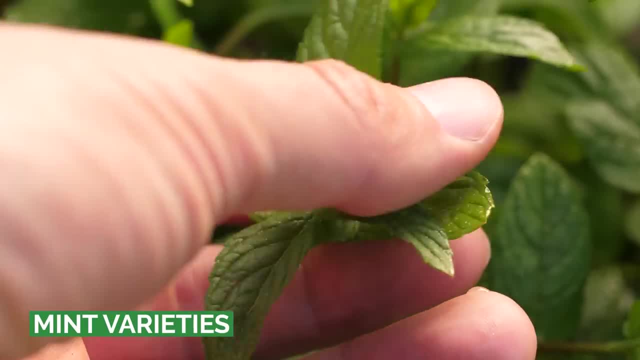 So just don't let it dry out. And now let's go through a little bit of the history of this plant and some of the coolest varieties you can grow. So mint is a fascinating plant. Its origins are somewhat unknown. It's kind of all around the world now and no one can really trace it down to one.